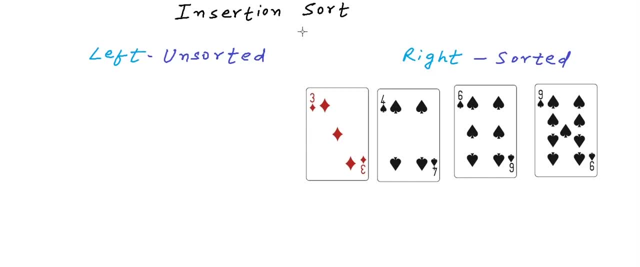 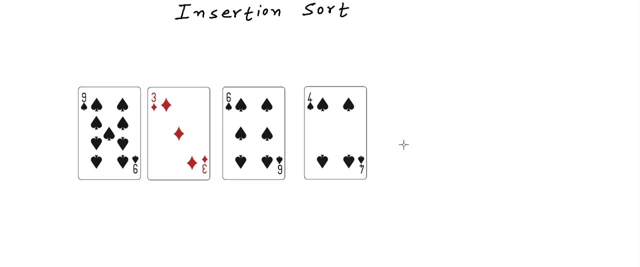 I have used two hands here, but if you see, this can be done in one hand also. The idea is pretty simple. What we are basically doing is we are dividing the set of cards into two subsets: A sorted subset or a sorted part, and an unsorted subset or unsorted part. Initially, all the cards. 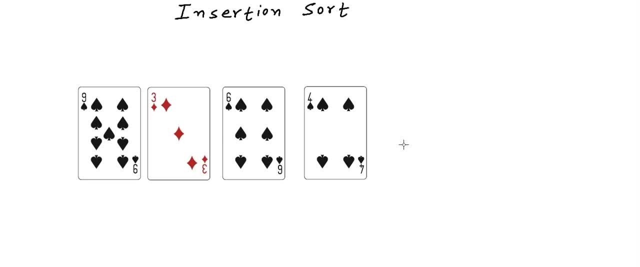 are in unsorted subset and the sorted part is empty and we are picking up one card from the unsorted part at a time and inserting it into the sorted part. Let's say we have something like this: we have a boundary here and, let's say, cards to the left of this line, this vertical line, are sorted. 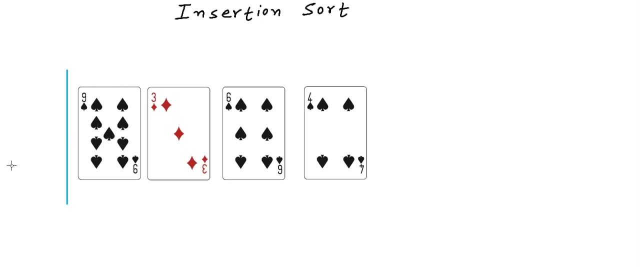 and cards to the right of this vertical line are unsorted. All the cards are in unsorted part. Now we will pick up one card at a time and insert it into the sorted part. If there is just one card, we simply move it. Now we pick up the next card. 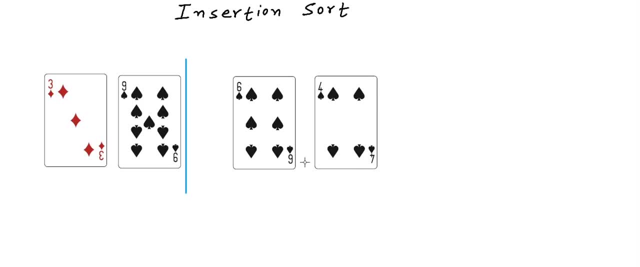 from the unsorted part. It's three. it will be inserted before nine in the sorted part. Now we will pick six, and six must be inserted between three and nine. And finally we will take four, and four must go between three and six. It should be inserted between. 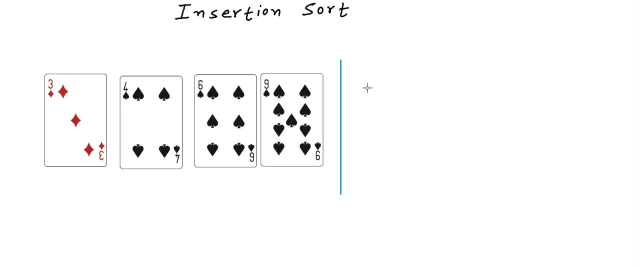 and six and we are done once our unsorted subset is empty. Now when we want to write a program to sort a list, we can do something similar to what we did for the cards. So let's say we want to sort a list of integers given to us in the form of an array. Let's name 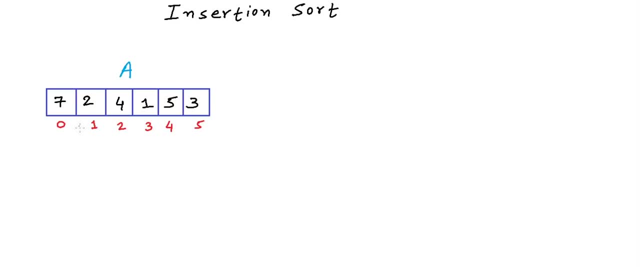 this array A. we have six elements in the array, So we have indices from zero to five. what we can do is we can start by saying that we will divide the array into two subsets. Initially, elements till index zero will be part of the sorted subset, or sorted half, because 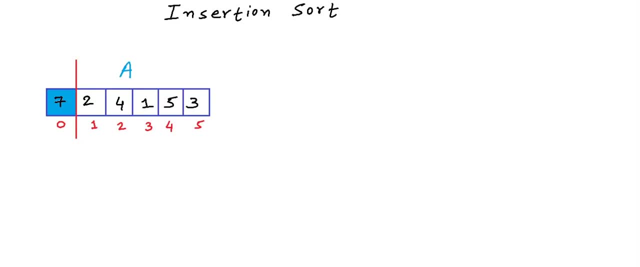 if you have one element in a set, the set is always sorted And all other elements are part of unsorted subset. And now we will go on picking elements from the unsorted subset And we will keep on inserting them into the sorted subset. So we will kind of keep expanding. 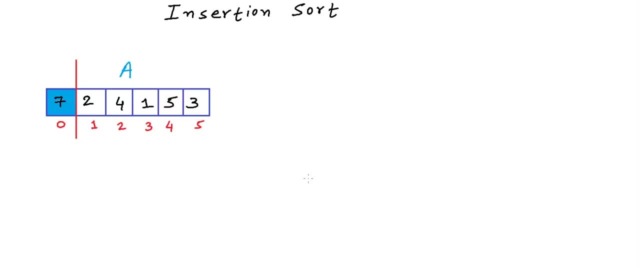 the sorted subset till unsorted subset becomes empty At any stage. let's say, the cells in blue Two are part of the sorted subset. Now, at this stage, I'll pick up two, which is the first element in the unsorted subset. programmatically, this will mean storing the value in some variable. 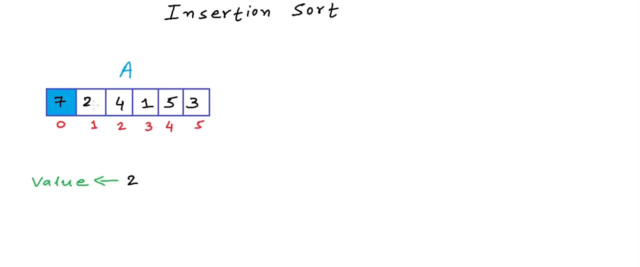 Let's say the name of the variable is value. So all we have done is we have said something like value is equal to a one, But for the sake of understanding, let's assume that we have taken out two from that position and we have created a hole there at that particular. 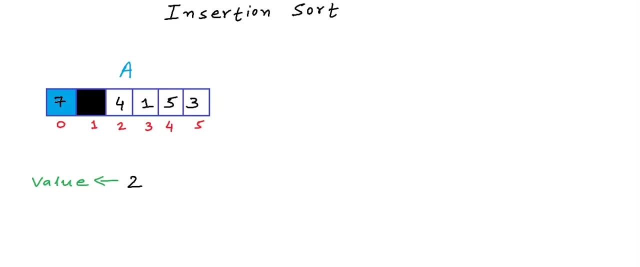 position. Now what we will do is to insert two. So if we insert two into the sorted subset, we will shift all numbers greater than two in the sorted subset by one position to the right. We have only one element at this stage in the sorted subset, seven, which is greater than two. So seven will be shifted one position. 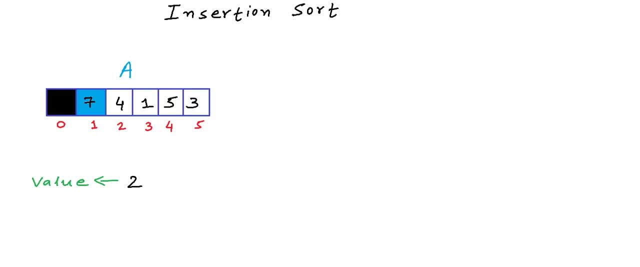 towards right and the hole will go to position zero, And now we will fill up two at position zero. we will fill up two in the hole, And now we are sorted till index one. Now, once again, we will pick up the first element from the unsorted part. So we will create. 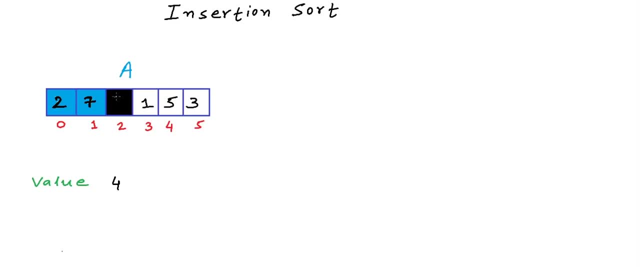 a hole like this. Remember, there is no actual taking out of four from this position. we are just filling up four in another variable and, assuming that there is a hole at that particular position, Now, once again, we will shift all the numbers greater than four by 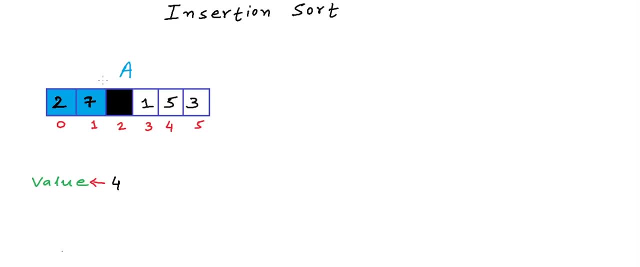 one position to the right. we will do so one by one. we will start at position one and see if the number is greater than four. seven is greater than four. So seven will be shifted to index two and the hole will now move to index one. Now we 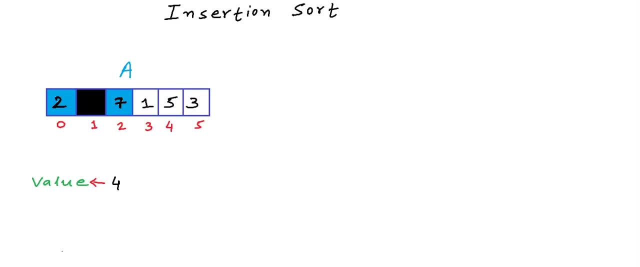 will look at two. two is not greater than four, So no more shifting is needed. we will simply put four at index one, And now we are sorted till index two, And now we will pick one from the unsorted part And once again we will start shifting all the elements greater than. 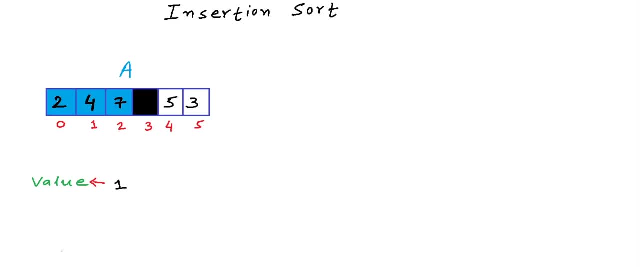 one in the sorted subset, one position towards right. seven is greater than one, So we will shift it and we will. the hole will now move to index two. number four is also greater than one, So it will also shift. number two is also greater than one, So hole will shift. 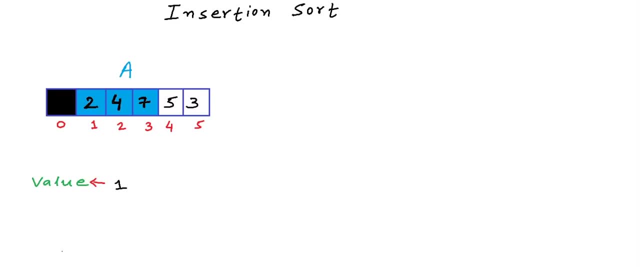 to zero And we do not have any more numbers greater than one to be shifted. So we will move one to this hole. And now we are sorted till index three, And we will repeat the same insertion logic for five and three as well. For five we will have to shift only seven. 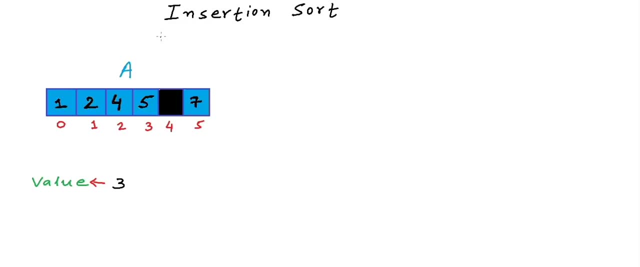 And for three we will have to shift seven, five and four, So finally three will go at index two. So finally we have a sorted list. This particular in place logic of shifting and inserting elements to sort a list is insertion sort algorithm. And now let's quickly write pseudo code for. 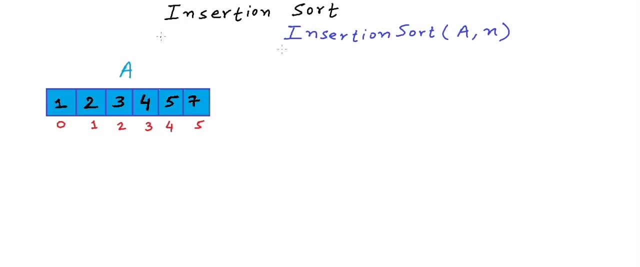 this algorithm. I'll write a function named insertion sort that will take two arguments: an array and the number of elements in the array. Let's say the name of the array is a and the number of elements in the array is n. Now, initially we are saying that we 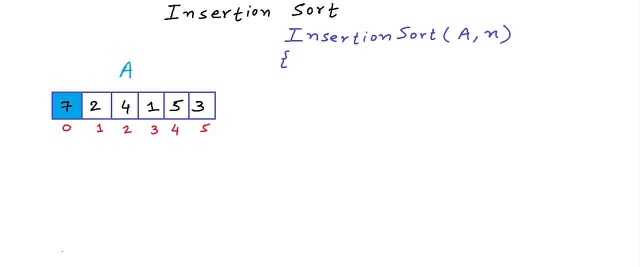 are sorted till index zero. So we will pick up elements from one till n minus one, And at each step we will insert the element at its appropriate position in the sorted subset. So in our code we will run a loop starting index one till n minus one, And first we will 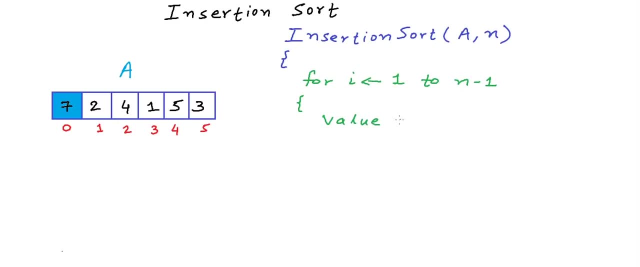 create a hole by by taking out the value to insert In another variable. so temporarily we will keep AI in this particular variable And then I'll take another variable to mark the position of the hole. At this stage, hole is at index i And now we need to shift all the elements greater than the value to be inserted one. 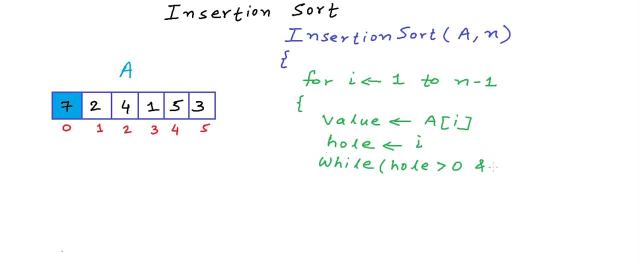 position to the right. while hole is greater than zero And and the element at index whole minus one is greater than value, we will shift the element at index whole minus one And the element at index whole minus one is greater than the value to the hole. So now our new. 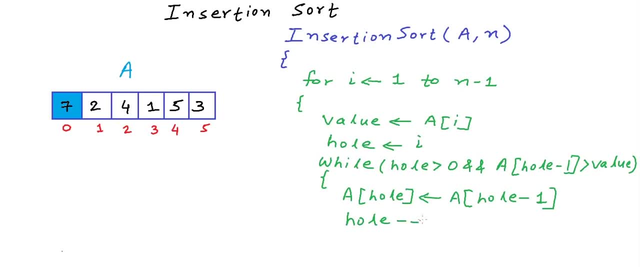 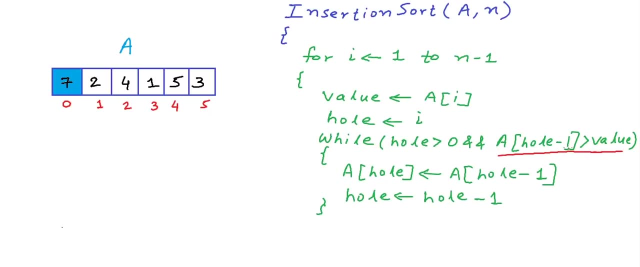 hole will be index whole minus one when we will find a smaller element than value in the sorted subset. So this particular condition will be false. we will exit the while loop. or we will exit the while loop when hole will be equal to zero. So there will be no more. 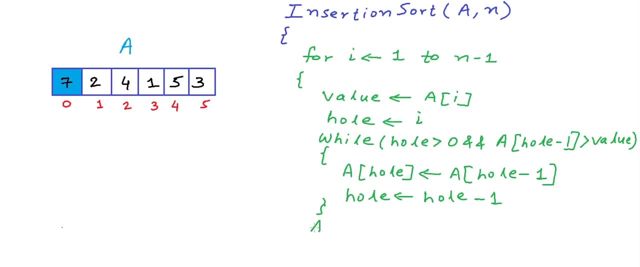 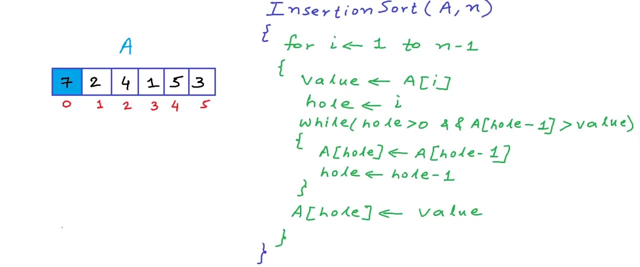 elements to shift. And finally, when we will come out of the while loop, we will put the value into the hole, And this is our pseudo code for insertion sort. I'll quickly walk you through this particular code and show a simulation with this particular example. 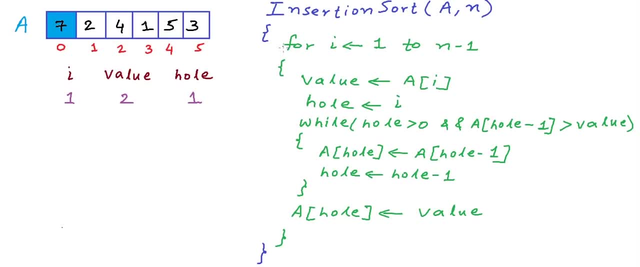 So we are running this code with this particular array. we will start with i equal one, so value will be two and hole will be index one. And now we come to the while loop hole is not zero, So we can be sure that there is an element before it and we can access the. 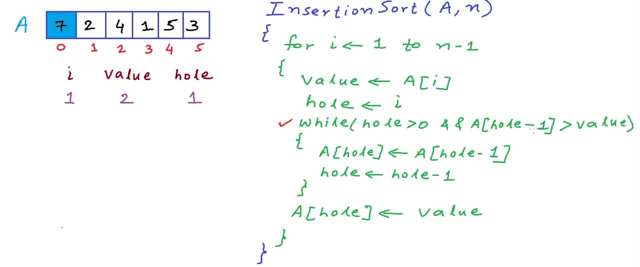 element at index whole minus one. whole minus one is zero And the element there is seven which is greater than the value two. I'll mark the hole with this color orange. And now we come here we'll say a hole in the element at index of whole. 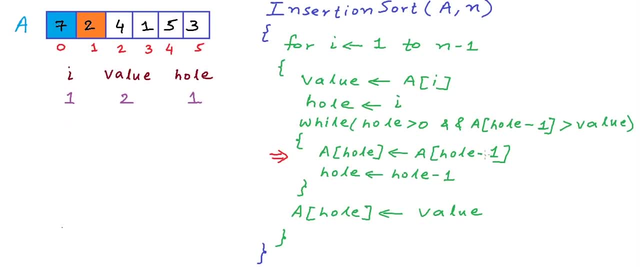 should be element at index whole minus one. So seven will now be written at index one and our imaginary hole will shift to index zero. And now, in the while loop, this condition will be false. whole is equal to zero. So we will come here, we will fill up two at. 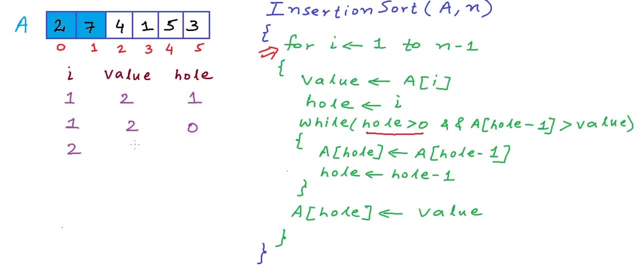 this particular position At index zero, and now I will be incremented, So value will be four and whole will be index two. seven is greater than four, So we will shift it and the imaginary hole will go to position one. And now a whole minus one, which is two, is not greater than value, So we will. 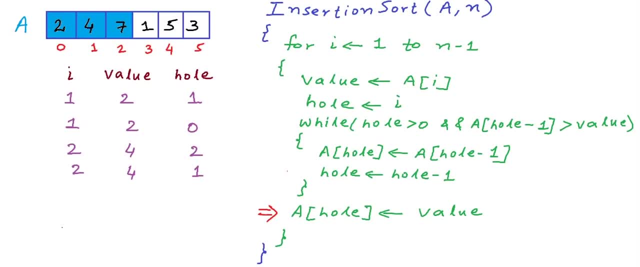 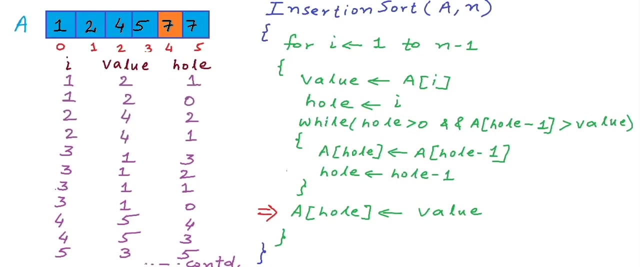 come out of the while loop and we will write four at this particular position And we will go on like this. For one, we will shift all the numbers And this will shift all the numbers in the sorted subset. So finally, we will have a sorted 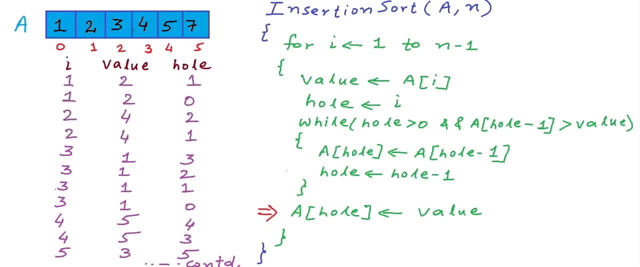 array. Sometimes the whole may not shift even by one position. we will not even go inside this while loop. in that case it will mean just taking out the value and inserting it again into the hole. it will happen when the number to be inserted will already be at its. 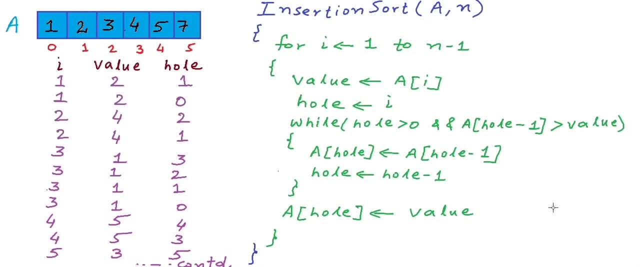 appropriate position. So this is pseudocode code for insertion sort algorithm for you. Let's now try to analyze the time complexity of this algorithm. We can try calculating the running time expression for this algorithm. Simple statements in a program execute in constant time. By simple statements we mean 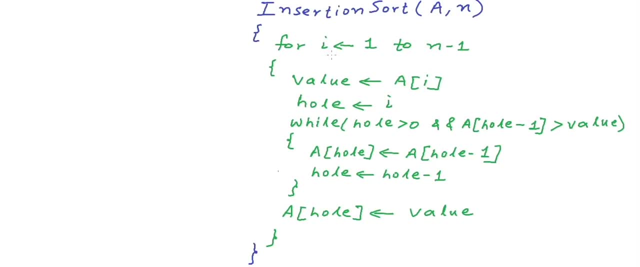 statements having simple operations like assignment, arithmetic or logical operations like these are simple statements. Let's say, these statements will take some constant time- c1, they'll together take some constant times. even these two simple statements will together take some constant time- c2.. And this particular statement will take some constant time- c3.. Now for our algorithm. 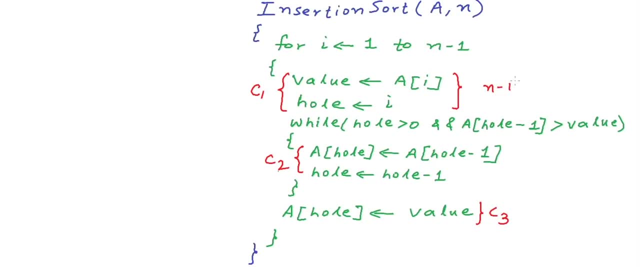 these two lines will always execute n minus one times. And how many times will these two lines execute inside the second loop? Well, it depends. it depends upon the input. when we will have a sorted array, then we will not go inside this while loop even once, because 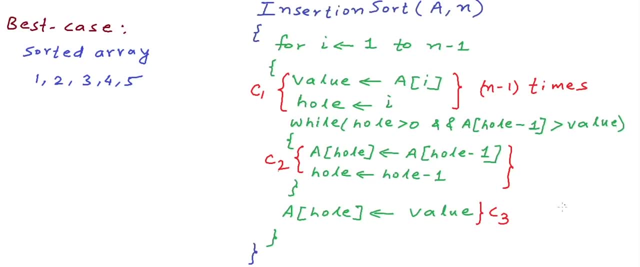 this particular condition will never hold true And this particular statement with cost c3 will also execute n minus one times. So overall time taken in the best case will be equal to c1 plus c3 into n minus one. there will be some additional cost to increment counters and all or to do this. comparisons inside this: 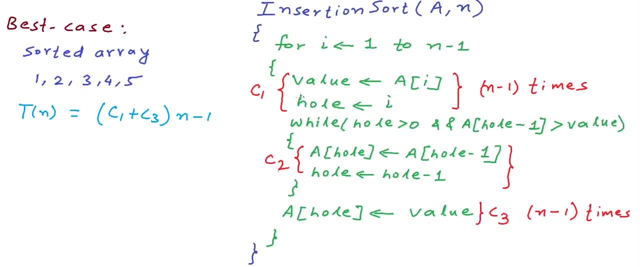 condition for loops. Let's assume that there are counted for in c1 and c2 respectively. Oh, this one should be n minus one in bracket. So we have a polynomial like a, n plus c2, plus b, where a and b are some constant in terms of c1 and c3. And whenever we have a, 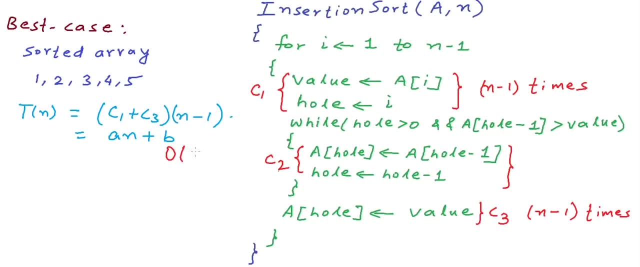 polynomial like this. for the running time it belongs to the set big O of the highest order term in the polynomial. So this will be big O of n. So insertion sort is big O of n in best case. we will have a worst case when we'll have a reverse sorted array, something. 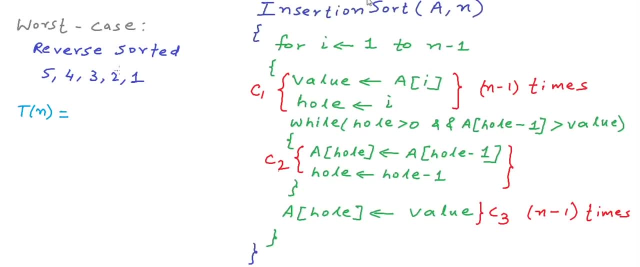 like 54321.. In that case, for i equal one, the statements inside the while loop will be executed once We will have one shift. for i equal to, we will have two shifts And we will go on like this. for i equal three, we will have three shifts, and for i equal n minus one, we will have